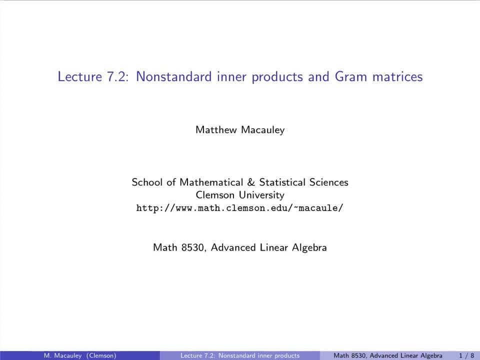 Welcome to Lecture 7.2, Non-Standard Interproducts and Gram Matrices. As a warm-up, consider an n by m matrix A over the real numbers where the columns are vectors x1 up to xm. The m by m square matrix A- transpose A is self-adjoint. We've already seen that. 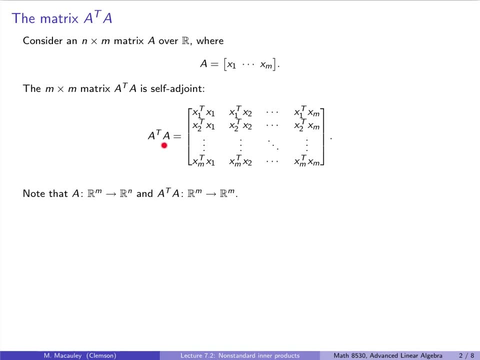 Remember that the ijth entry of A transpose A is xi transpose times xj. So you can really think of this matrix as the matrix of dot products, of all pairs of these vectors. xi Recall that A and A transpose A have different domains, So A goes from am to an, whereas A transpose A goes from am to an. 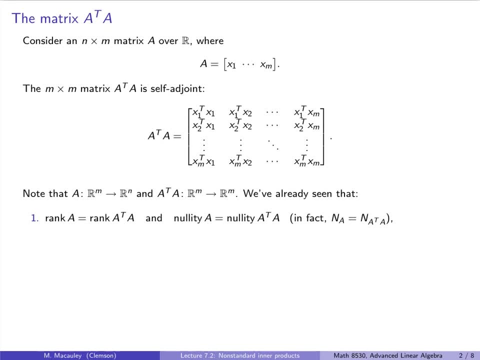 Let's summarize a few important points about the matrix. A transpose A, First off A and A transpose A have the same rank and the same nullity. Even more than that, they actually have the same null space. So not just the dimension is the same, but the actual null space is the same. 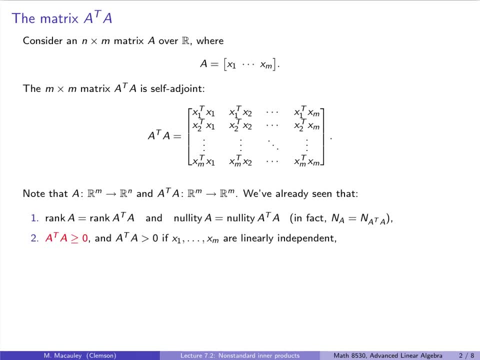 We've proven that. We've seen that A transpose A is non-negative And it's positive if the vectors x1 up to xm are linearly independent. We've seen that if the null space of A is trivial or equivalently if the columns are linearly independent. 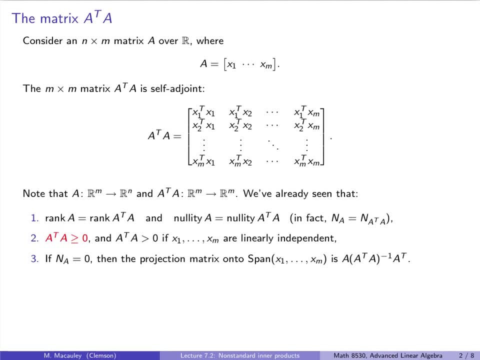 then the projection matrix onto the span of those columns is A times A transpose A. inverse times A- transpose. Later in this section we will diagonalize A transpose A to get the celebrated singular value decomposition of A which comes up in many applications in applied math and statistics. 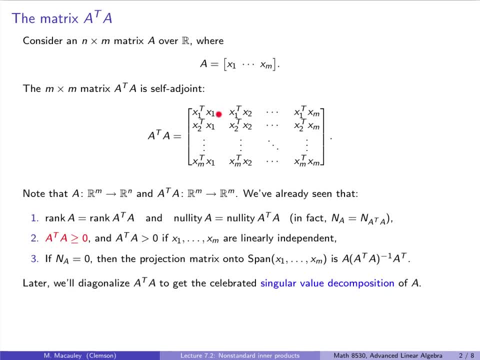 So the takeaway here is that this is a very important matrix. It can be really thought of as the true way to square a matrix, And when I say that I mean you could of course square a matrix, but you might get complex or negative eigenvalues. 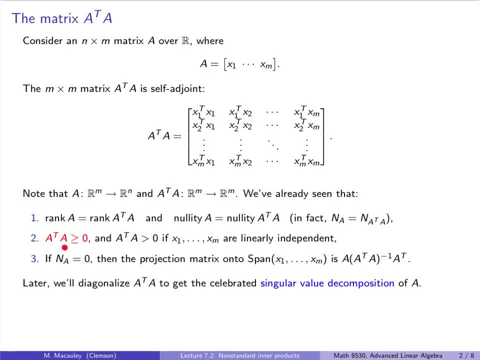 This is why you get a matrix that's not a square matrix. This is why you get a matrix that's not a square matrix. This is why you get non-negative eigenvalues, And one reason why it's so important. well, in addition to this first property, 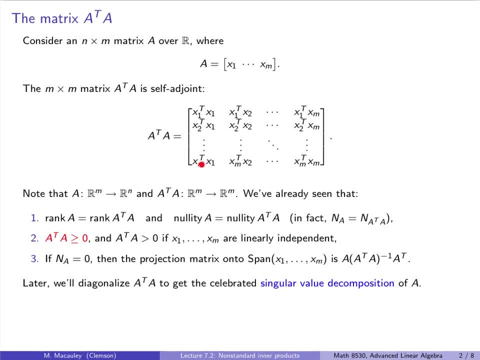 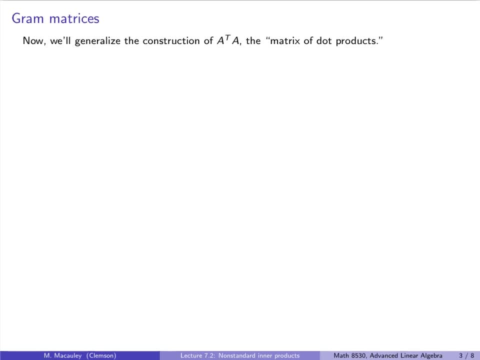 really why this holds is because it is the matrix of all dot products And that's what we are going to generalize in this lecture. So let's do that now. We'll generalize the construction of A transpose A, which you should be thinking of as the matrix of dot products. 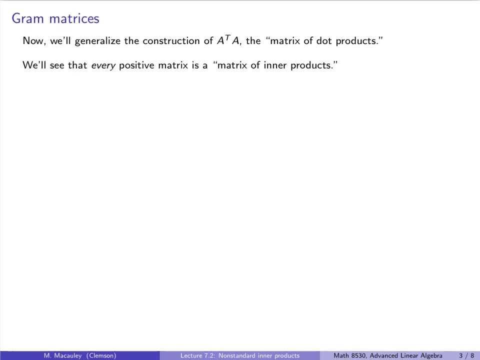 We'll see that every positive matrix has this form can be thought of as a matrix of inner products, for some vectors and for some inner product structure, And this is perhaps a little surprising, because the property of being positive does not depend on the inner product structure at all. 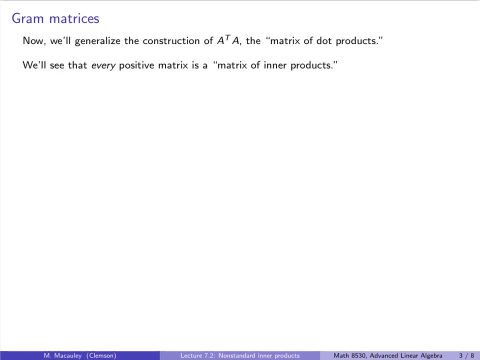 It actually depends just on the structure of the linear map because it depends on the eigenvalues. But the matrix of inner products depends on both the choice of basis and on the inner product structure. It's time for a definition. The Gram matrix of m vectors x1 up to xm. 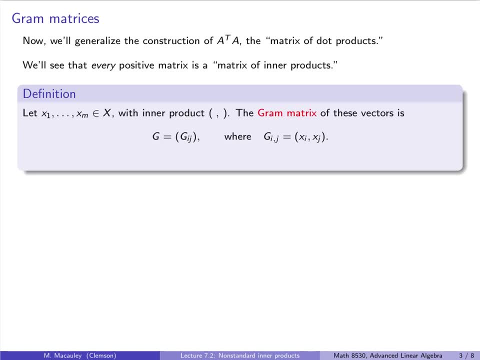 is the m by m matrix, where the ijth entry is just the inner product of xi with xj. Notice that g is simply the matrix A star A, where A is the matrix whose columns are x1 up to xm. Let's now prove what I've basically already claimed. 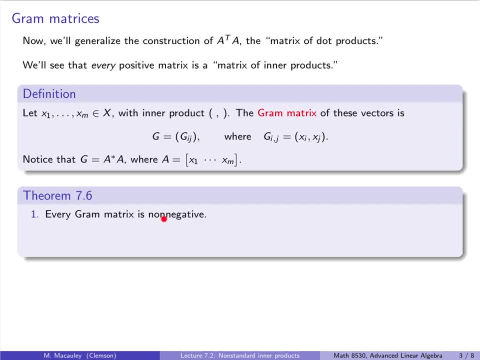 First off, that every Gram matrix is non-negative. So there's nothing special about A transpose A Here we just used the standard inner product. But remember that if we pick an orthonormal basis, then any inner product we deal with can be written as dot products. 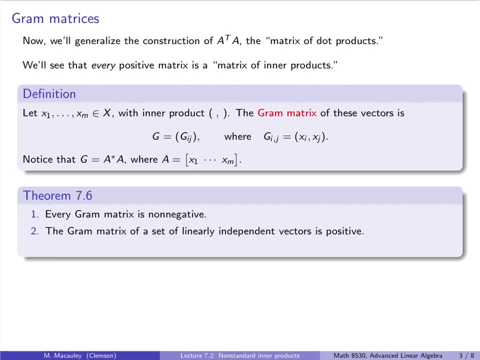 Next, the Gram matrix of a set of linearly independent vectors is indeed positive, just like what we had for A transpose A. And finally, every positive matrix is a Gram matrix. So what we will do is, given a positive matrix, we will show how to. 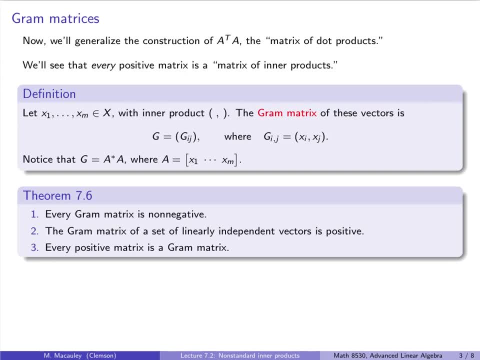 construct an inner product, a new inner product, so that this matrix is the Gram matrix of a collection of vectors. Let's get started with that right now. Let's prove this now. In fact, we can do 1 and 2 together in. 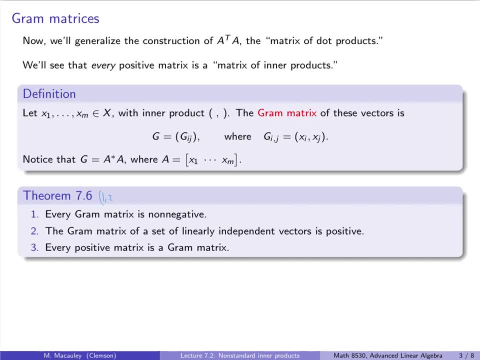 basically one line. except that line is going to be a little bit notationally messy And because of that it's going to hide some of the intuition. So I'll do that line first and then I will unpack it and draw it in. 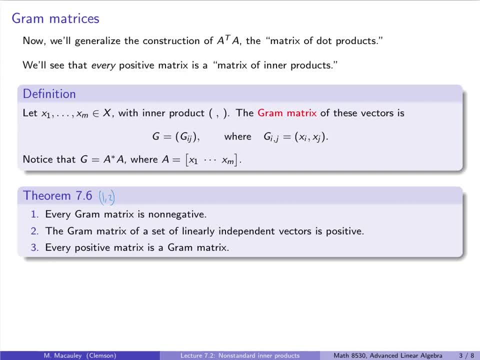 matrix and vector form so you can really understand what's going on. So let's take a vector, z, and we need to show that the inner product of z with gz is non-negative. So remember, let me write it up here: inner product of z with 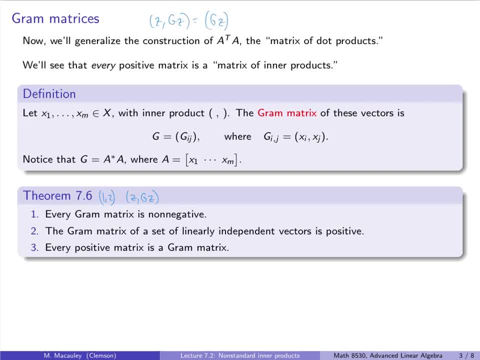 gz. that is gz conjugate transpose times z. So that's z conjugate transpose g conjugate transpose times z. So if we write this out, this is the sum over all over n squared terms of the form zi times gij bar. 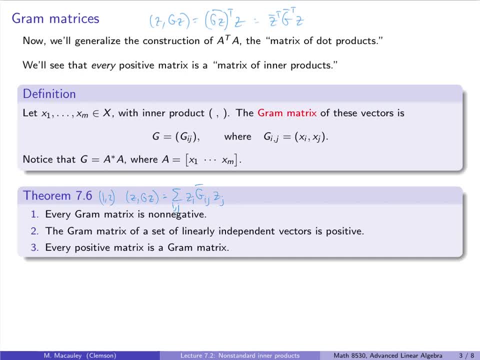 times zj bar. And so, by definition of this matrix, I'm just going to plug in what this is. This is the inner product of xi, xj times, zi times zj bar. So, again, this is the sum of n squared terms. 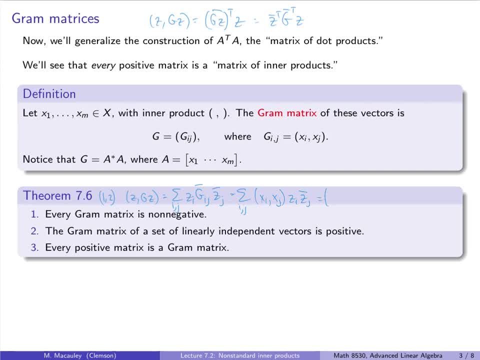 but we can write it as an inner product of two vectors. i equals 1 up to m of. I have to be careful here. this is zi. these are the coefficients times xi, and the sum from i equals 1 up to. 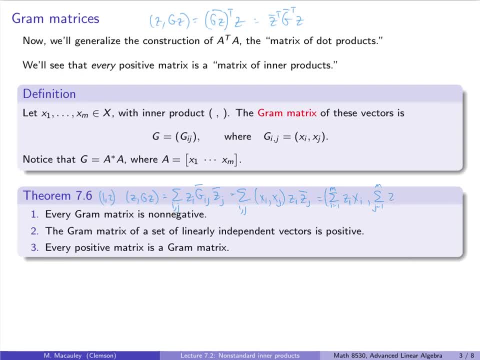 m of, or actually I'll call this j? zj times xj, And this notice- is the norm squared of this vector. So j equals 1 up to m zjxj, And that is automatically going to be non-negative. 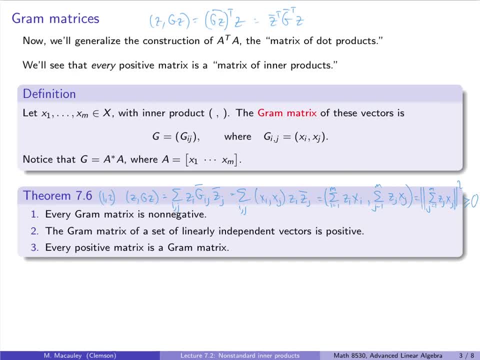 And, moreover, if the xi's or the xj's are linearly independent, then this is going to be a. this is not the zero vector, so it's going to be strictly bigger than zero. So that's why the grand matrix. 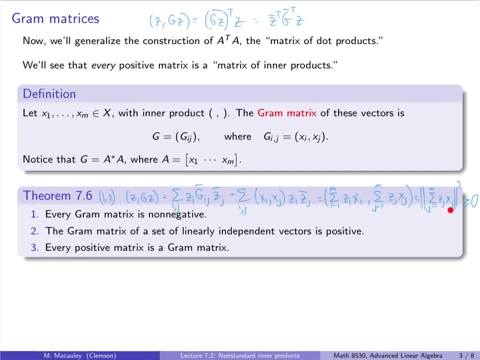 is positive if the xj's are linearly independent. So it, if you believe this. we've proven 1 and 2.. But you know, whenever you have these double sums and these double subscripts, it's not you really have to pause. 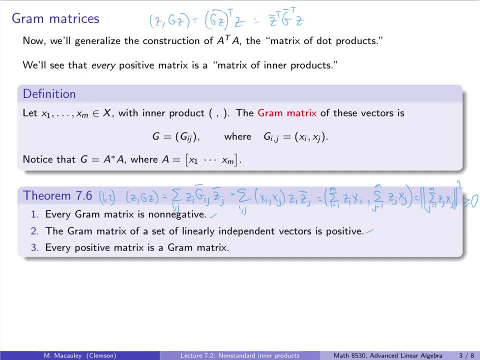 every single step so you can verify that and you don't really get the full intuition. So that's what I want to do now. So what is this really saying? So let's write this in matrix notation: So g, so z. 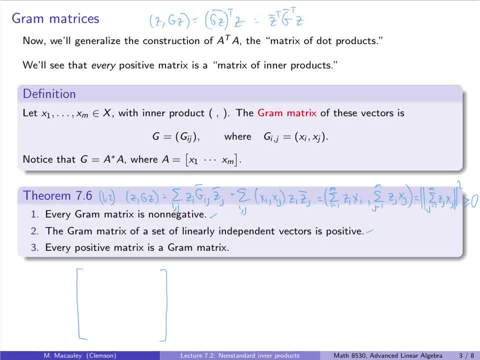 the inner product of z with gz. I'll write it like this: So this is z1, z2, up to zm, And then what I have here. I have z1, z2, up to zm, And I really should put bars here. 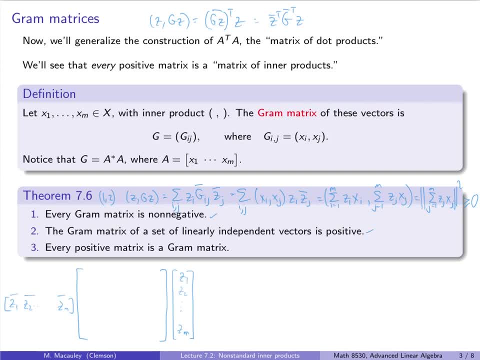 And then the entries here are of the form. so this is x1, x1, x1, x2, up to xm- xm, And down here we have xm- x1, all the way up to xm- xm. So we have this matrix. 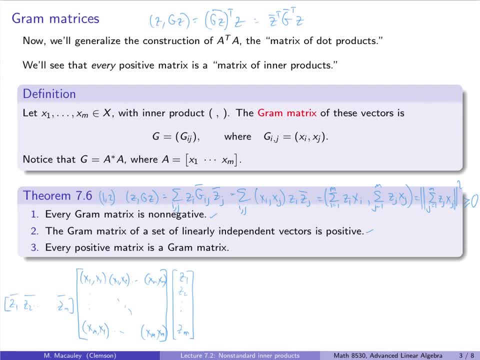 And it's not clear what to do with this, how to get this norm squared here. So what I'm going to do is start here and work backwards And kind of meet in the middle. So now maybe this notation can be improved. but 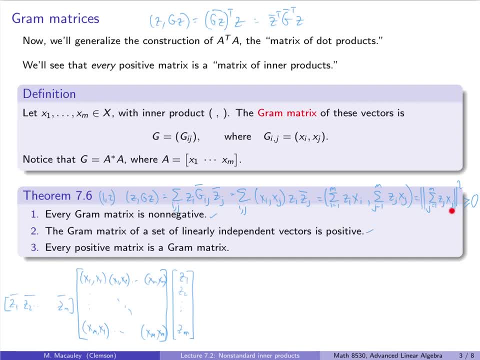 the zj's are coefficients and the xj's are vectors. So this, so clearly, this norm squared is just this inner product. so let me expand that. I'll do that down here. So this is z1, x1,. 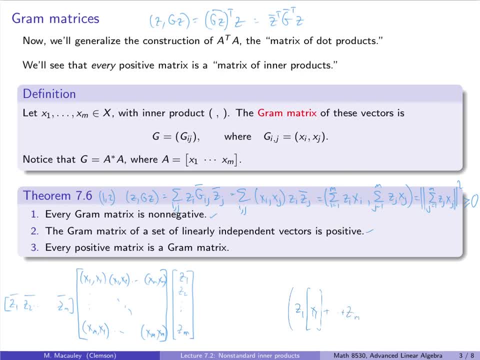 plus dot dot dot zm xm, The inner product of that with itself. So z1, x1, plus zm xm. And if I were to give you this and I say, how would you evaluate it? Well, you use bilinearity. 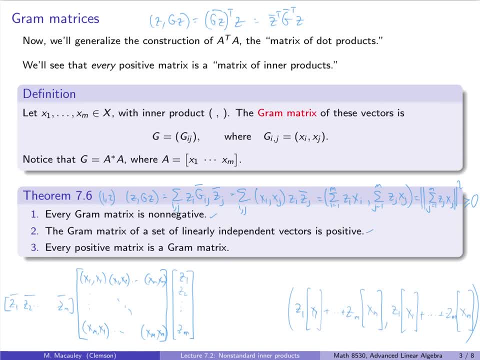 and you break this up into n squared terms And the terms are going to be the inner product of zi xi, with zj, xj, And, using the definition of the inner product, what we are going to get is zj. 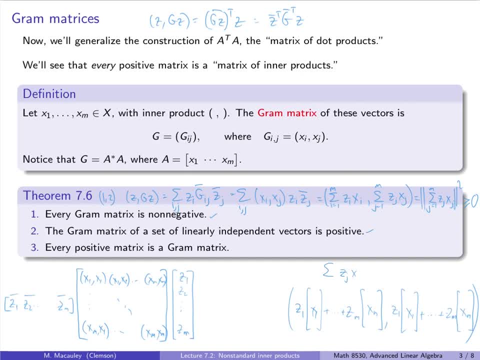 xj. These are bars And this should be a transpose with zi, xi. And again, these are vectors and these are scalars. But notice that that's really what I have here And I don't think it's a stretch to see why. 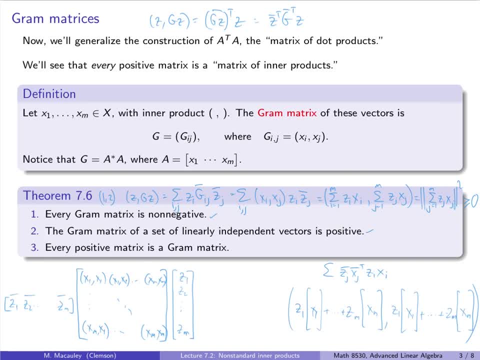 that's exactly what this is as well. So again, I haven't proven it completely this way, but I did this one line proof And I think you can see the intuition as to what's going on when you write it in matrix notation. 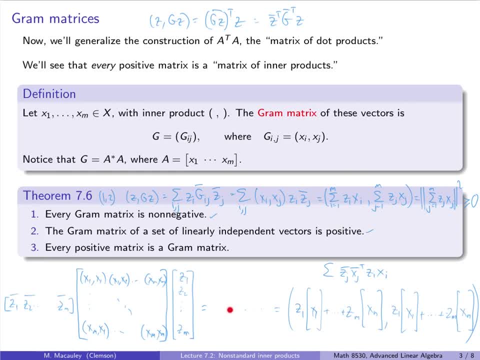 Because we start out with this and we end up with this, And it's not too hard to fill in these gaps. Finally, for part three, before I do it, let me give you the intuition. So I'm going to write a matrix. 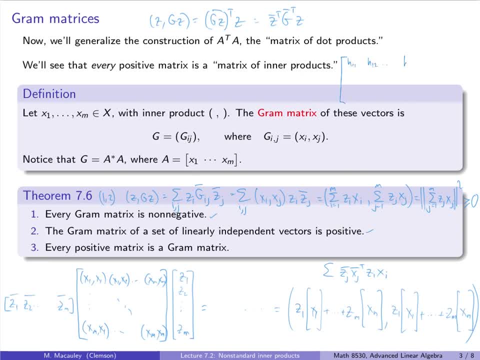 H11,, H12, H1M. Say: this is an arbitrary positive definite matrix, So this is HMM And this is HM1. And so forth. Now look what happens if I multiply here by the jth unit basis, vector ej. 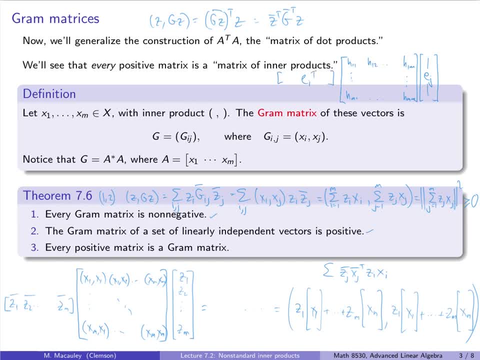 And then ei transpose. So if I do that, I literally just pick off the hij entry. So I'm going to define an inner product, So the inner product of ei and ej, if I can define an inner product where this is hij. 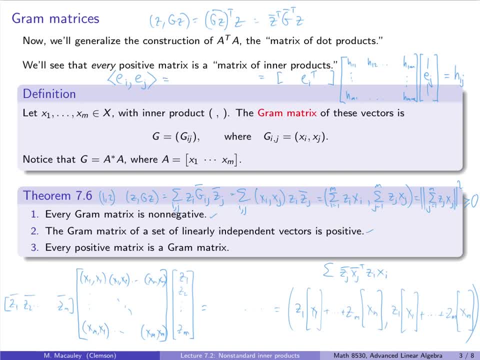 then I'm done. So I will define what I call the non-standard inner product of ei and ej to be based on my default inner product, The inner product of ei and hej, Because h is self-adjoint and positive definite, this is an inner product. 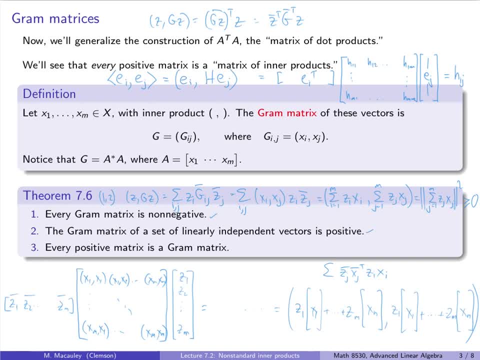 And I claim that in this case, the inner product of ei and ej is indeed hij, And I'll let you check that using this definition, And it may look like that I put the the. using this definition, you say, well, the ej should be over here. 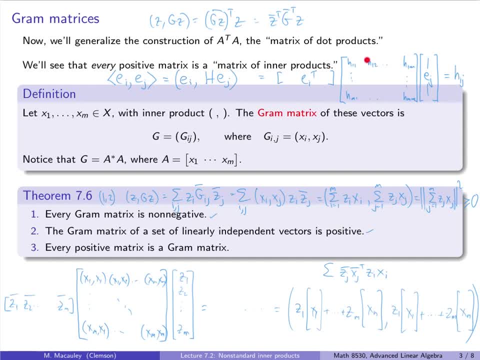 and the ei should be over here. That is true, but then we have to take the conjugate transpose of this as well, So this is indeed equal to hij. So, given an arbitrary positive matrix, we have defined an inner product. so which um? 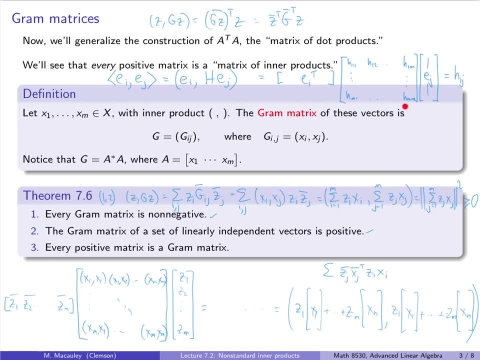 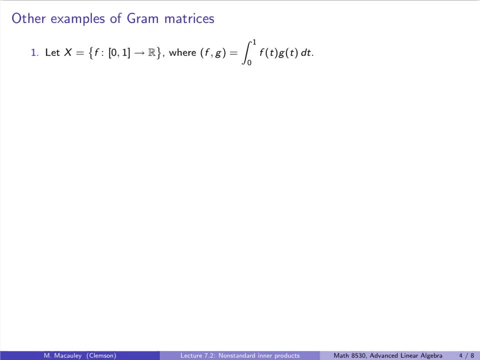 and with respect to this inner product. this matrix ei is our matrix of dot products Or our matrix of inner products. Now, for fun, I want to show you two examples of gram matrices that arise from vectors in infinite dimensional spaces of functions. To begin, 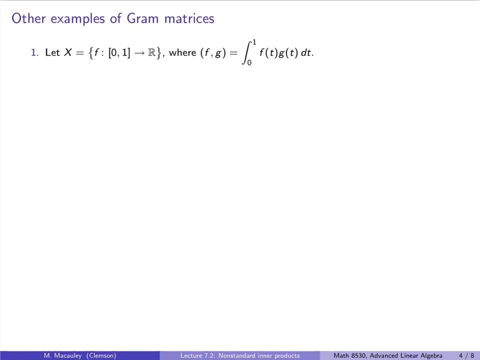 let x be the space of real valued functions on the interval where the inner product of f and g is just defined to be the integral of their product. on zero to one, If we take the m vectors, that are the smallest powers of t. so t to the zeroth, t to the first, up to 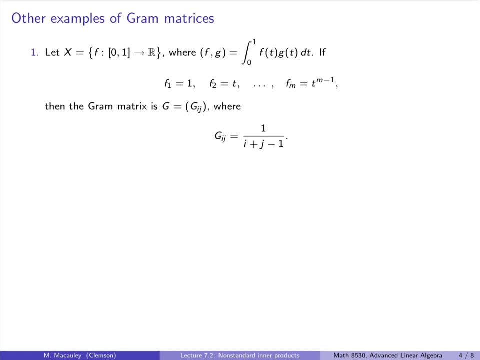 t to the m minus one, then the corresponding gram matrix is g, where the ijth entry is easily computed by just integrating t to the i minus one times t to the j minus one, zero to one, and a very simple calculus exercise gives us that that is one over. 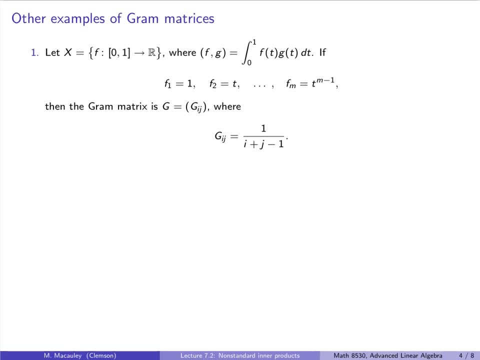 i plus j minus one. For a more familiar example, consider the space of complex valued functions on zero to two pi. If you prefer, you can think of these as periodic functions on the real line. And let w be a weighting function, so a positive. 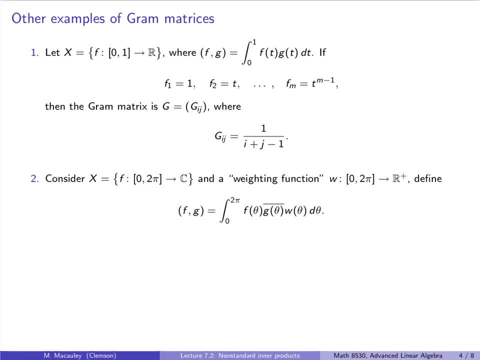 function on zero to two pi. Let f be the integral on zero to two pi of f of theta, g of theta bar times w of theta d theta. If fj is the complex exponential, e to fj is the generalization of this the j theta. for well, let's take finally many of them. so let's say j equals negative n. 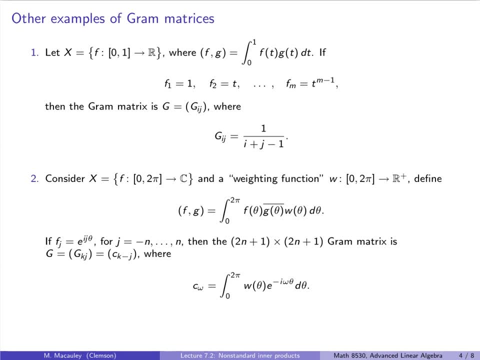 to positive n. so this isn't here. we have 2n plus 1 vectors, so the gram matrix is 2n plus 1 by 2n plus 1, and I don't want to call the entries gij again, because i is now the. 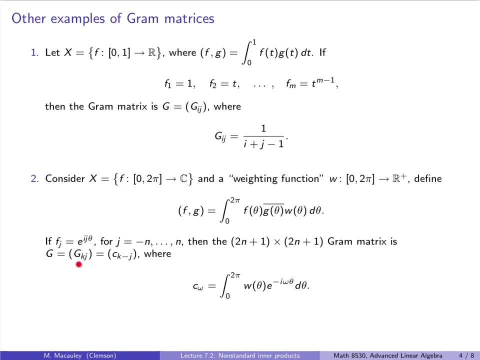 square root of negative 1, so let me call it gkj. and so the kjth entry is a Fourier coefficient, namely ck minus j. and remember that formula for a Fourier coefficient, c, omega, is the integral from 0 to 2 pi of omega, of theta e to the negative i. 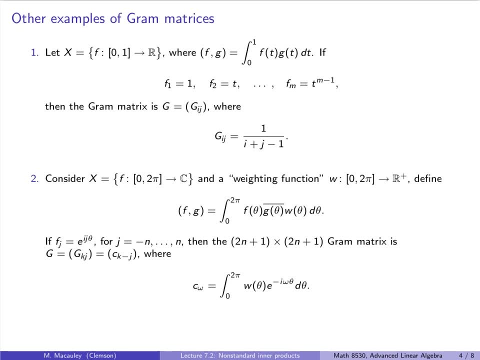 Okay, so if you want to know more about this- there's a lot more I could say about this- I would actually encourage you to go back and watch that video on generalized Fourier series and stromal level theory. Moving on, I want to revisit this idea that we talked about earlier. 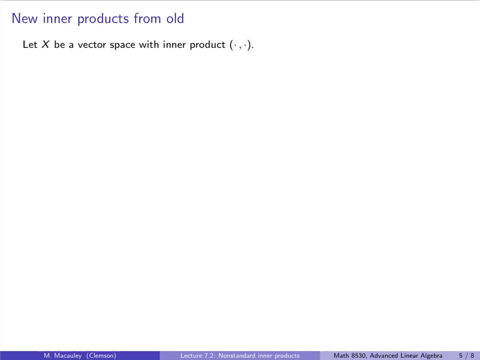 Did a couple slides ago about defining a new inner product using a positive definite matrix. So if x is a vector space with inner product, that I will denote with parentheses. a positive map m defines a so-called non-standard inner product that I will use with angle brackets. 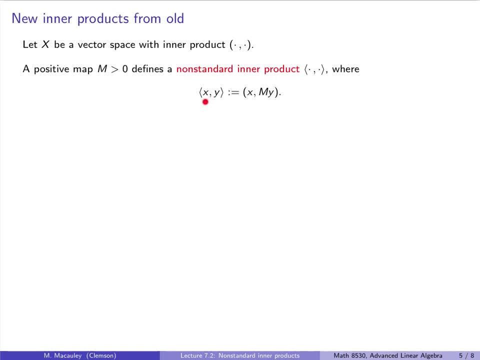 defined as follows. So the new inner product of x and y is the. Now, I've done examples like this previously in the course. I just haven't called it this because I didn't really have a use to call it this until this lecture, when we wanted. 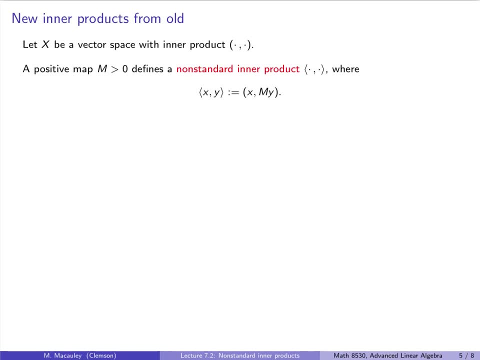 to prove that every positive matrix is a gray matrix, and we're going to continue with this. But first I really want to emphasize an important point, and that is that being self-adjoint is a property of the inner product. So there's going to be linear maps that are self-adjoint in one vector space or one inner. 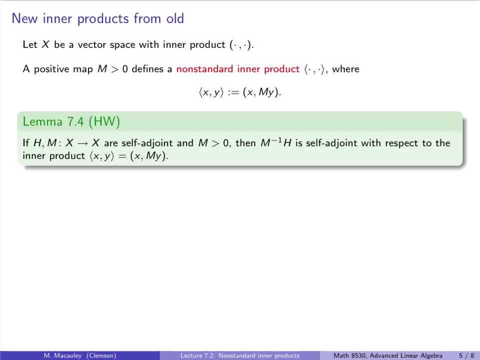 product space but not in another, or vice versa. So here's a lemma I said is a homework. I think I'll do it because it's very simple. So if h and m are self-adjoint with respect to some inner product and m is positive, 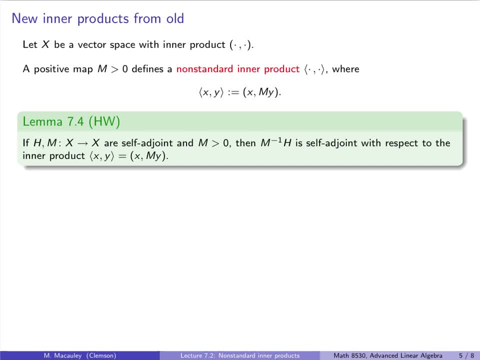 then m inverse. h is self-adjoint with respect to the non-standard, And to see why this is, it basically follows pretty simply: Let's write out what. so for this to be self-adjoint, let's write the inner product of x and m inverse. 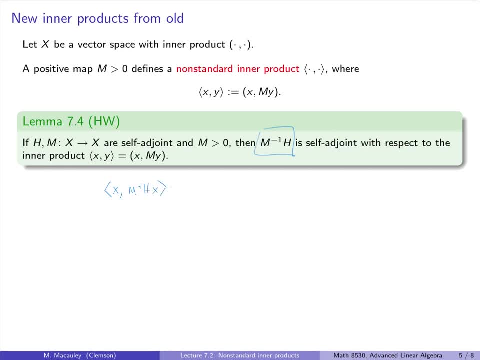 h x. and let's go back to our standard inner product. so x dot m times m inverse h. Of course this cancels to get inner product of x at h x. And now let's see for this to be self-adjoint we have to put it in the left coordinate. 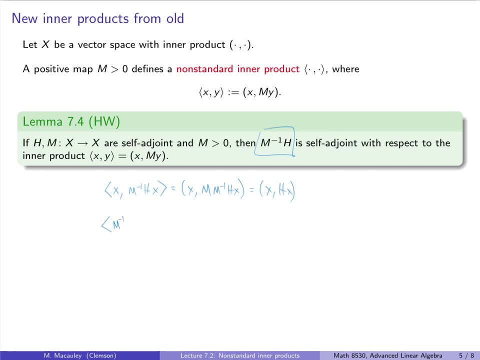 and see that we get the same thing. So m inverse h x. dot x in our non-standard inner product. Let's bring it back to our standard one. So that's m inverse h x, m inverse h x. Let's go back here. 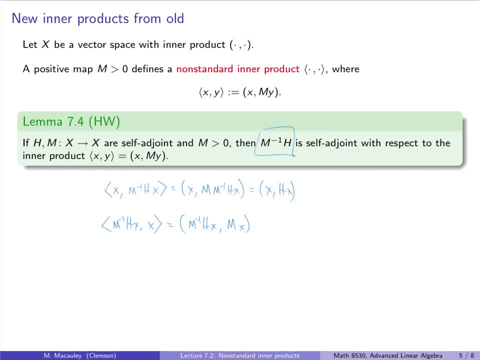 And see that we get the same thing, m, x. and if m is self-adjoint then we can move it over here and get m? m, inverse h x, dot x or just the inner product of h, x and x. 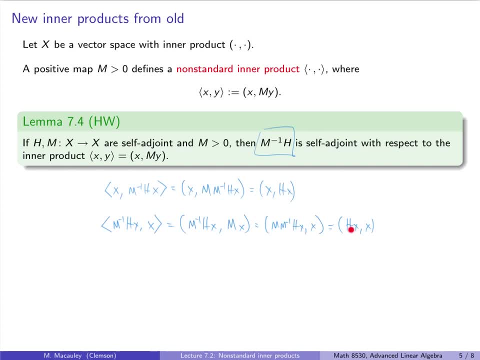 And we know that these two are the same because h is self-adjoint. Let's explore this a bit further. If being self-adjoint depends on the inner product structure, that means we can probably find a linear map that's self-adjoint with respect to one of these but not the other. 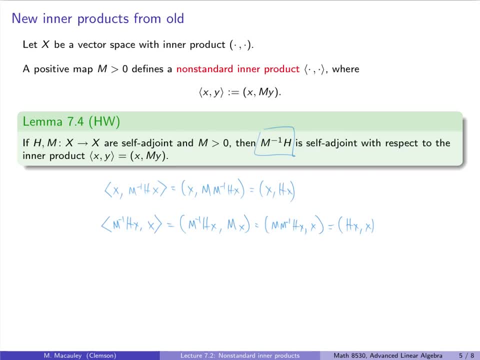 And so let me just take h, which is self-adjoint with respect to the standard inner product, And I claim that h is probably not going to be self-adjoint with respect to this non-standard inner product- And let's explore. 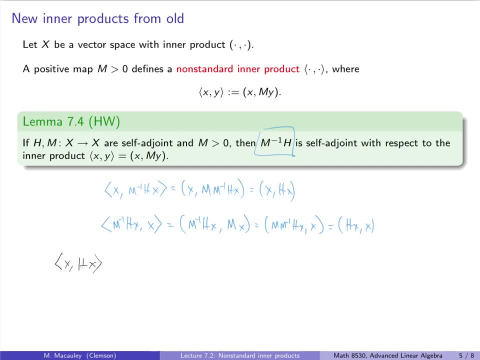 So x, dot, h x. the new inner product is the old inner product of x, dot, m, h, x, and if we put h in the other coordinate we're going to get h, x, dot. x equals parentheses, h x. 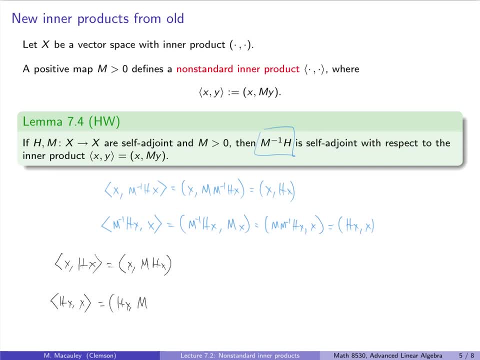 dot m, x. And now, if m is self-adjoint, we can, so m and h are self-adjoint, so I can move m over here. Actually, let me move h over here, and I'm going to write this as inner product of x. 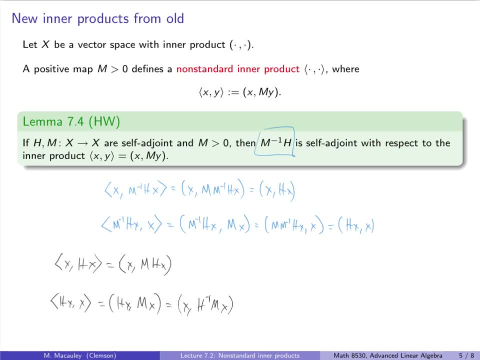 with h inverse m x, and it's generally not going to be true that m h is equal to h inverse m. So if you find any matrix A for which this does not hold, then h is not going to be self-adjoint. 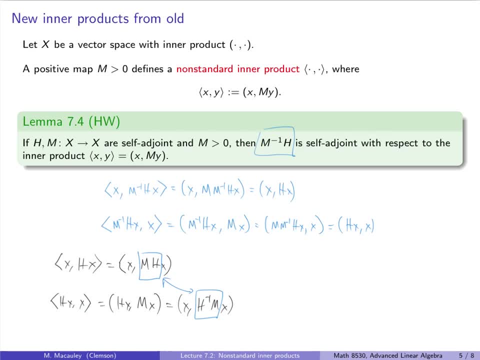 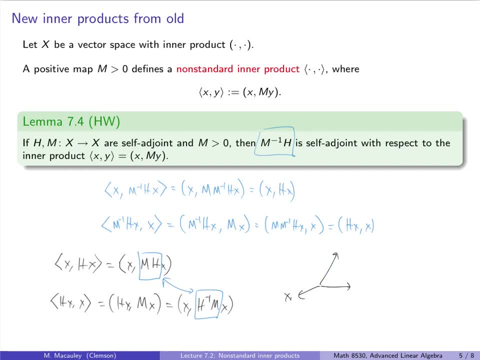 like this: say x1, x2, and x3. So if these are not orthogonal with respect to the standard dot product, then that matrix is not going to be self-adjoint or symmetric. However, we can certainly define an inner product structure. 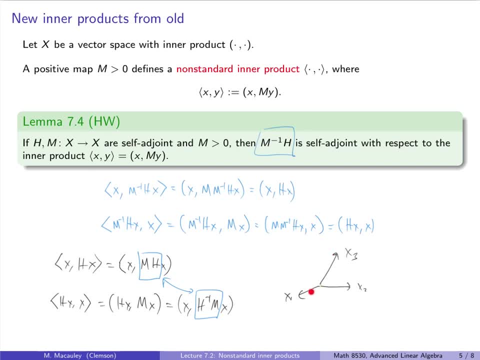 where these vectors are going to be orthogonal And in that case, with respect to that inner product structure, the matrix is going to be self-adjoint, Because remember the way to think about what a self-adjoint matrix is. I've said this multiple times and I will continue to say this. 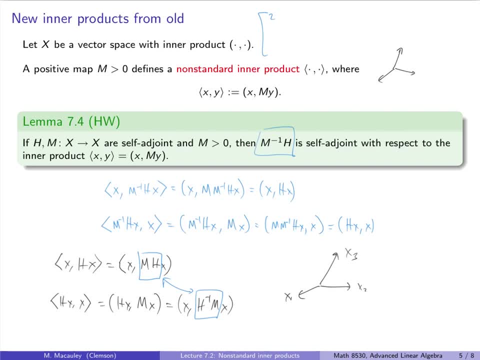 is if you tilt your head in the right direction. think of the linear map: 2,, 3,, 4,, the diagonal matrix: it stretches this direction by 2,, this direction by 3, and then this direction by 4.. 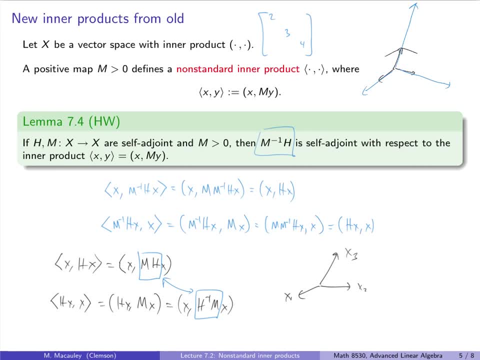 In other words, it sends the unit cube to a rectangle or, sorry, a box, a rectangular box rather than some parallel pipette. So when I'm saying rectangular versus parallel pipette, I'm saying any two of these vectors are going to be orthogonal. 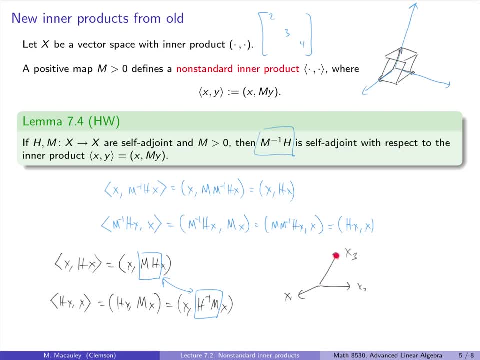 and that depends on the inner product. So even if to our standard Euclidean eyes, if this looks like it's not orthogonal, if you put a geometry on it where these things are orthogonal, by finding the correct inner product space. 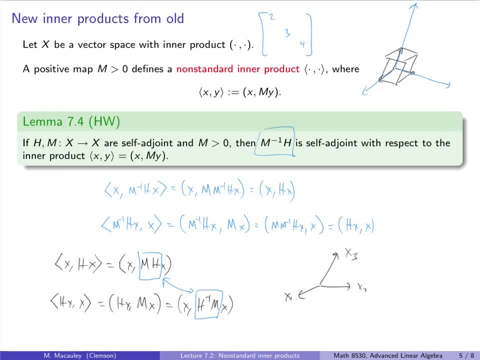 then when you apply the linear map, you're just, if these are the eigenvectors, you're just going to stretch these out or squash them by something and just geometrically you can see that what you're doing is what I'm describing up here. 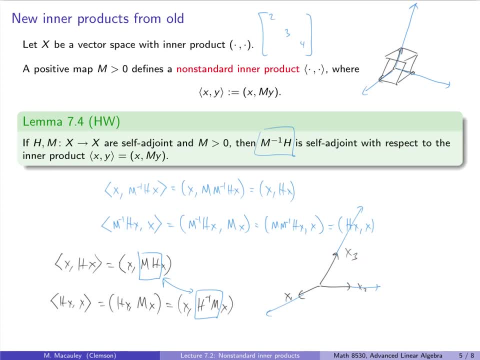 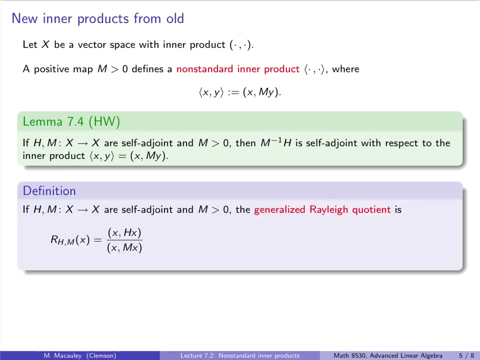 with a different geometry. So this is a self-adjoint map with respect to that new inner product. So takeaway message is that the property of being self-adjoint-ness is dependent on the inner product structure. Moving on, let's continue with self-adjoint maps H and M. 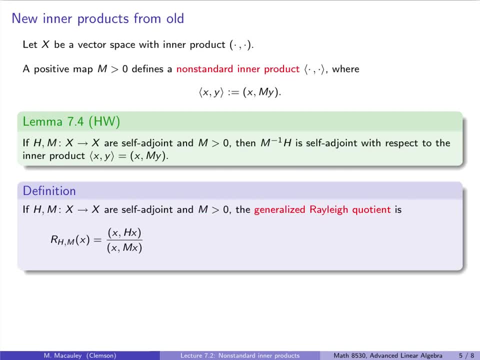 and positive M. We can define the so-called generalized Rayleigh quotient to be R sub H comma M of X, the quotient of the inner product of X and HX with the inner product of X and MX. Now this may look a little bit weird. 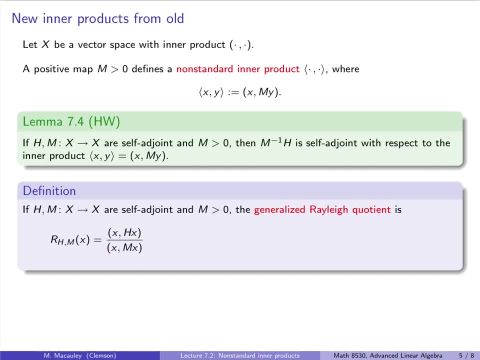 out of left field. but let's work with it a little bit. If I rewrite this by sticking in an M- M inverse up here, then I can rewrite this with a non-standard inner product, namely the inner product of X and M inverse HX. 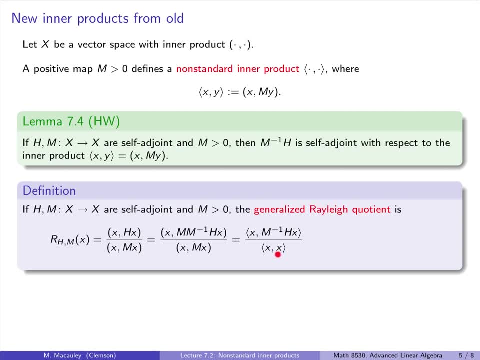 over the inner product of X with itself, with the non-standard inner product, And this is just the Rayleigh quotient of M inverse HX with respect to this inner product. So, in other words, the generalized Rayleigh quotient is a standard Rayleigh quotient. 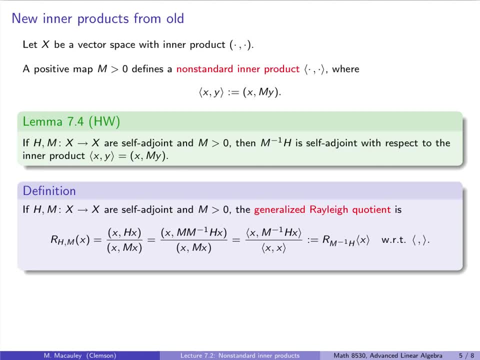 in a different inner product space. So this is very non-standard notation, but to distinguish between the two inner product spaces, instead of using parentheses to denote the argument, I'm going to use angle brackets like this. Now, another possibility is to put the angle brackets. 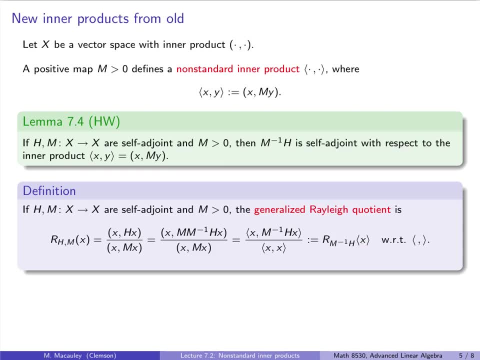 or the parentheses as a superscript, but I think that just gets too messy. I like it, like this. So several easy comments. The ordinary Rayleigh quotient is simply the generalized Rayleigh quotient with respect to the identity map. And next, something I just said. 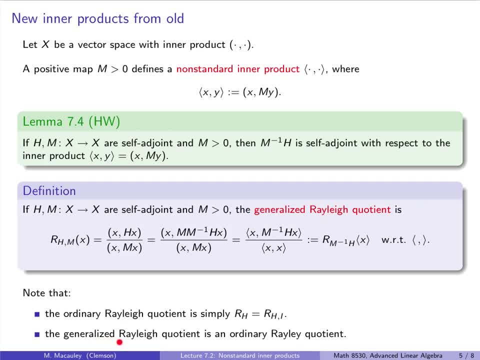 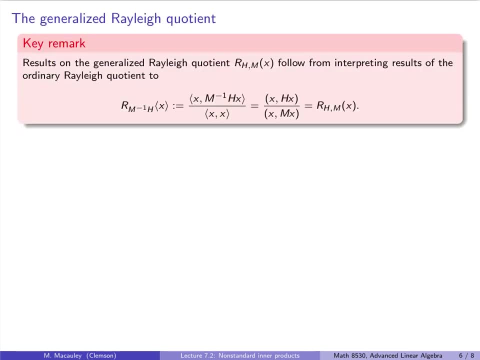 but I want to emphasize: the generalized Rayleigh quotient is an ordinary Rayleigh quotient, just with a different inner product structure. What this means is that all of the results that we have proven for the ordinary Rayleigh quotient carry over to the generalized Rayleigh quotient. 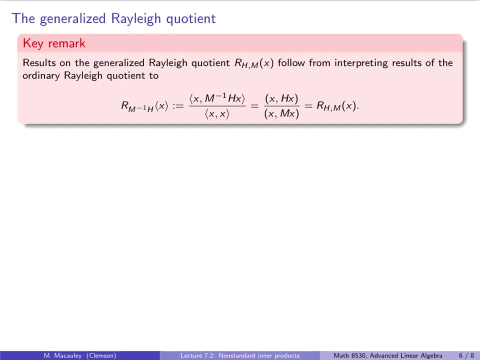 We just have to interpret them in the right inner product. So I'm going to go through and resummarize them. Please watch the video on the Rayleigh quotient if you have not already. otherwise this is really going to come out of left field. 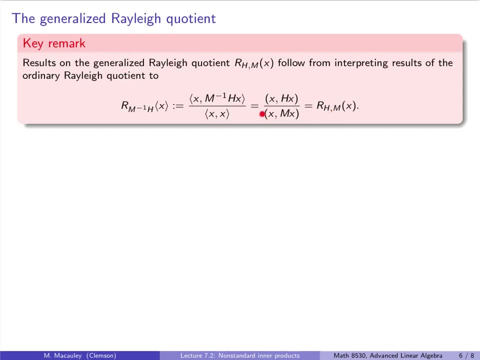 So, once again, this is just the definition. I'm writing it up here for reference for what I'm going to show you next. So the minimum value of the Rayleigh quotient is the smallest eigenvalue. So for the standard Rayleigh quotient, 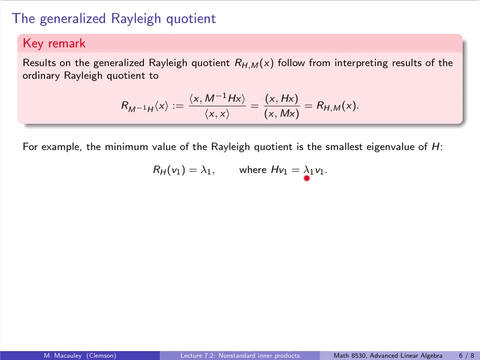 it's lambda 1, where hv1 equals lambda 1v. The generalized Rayleigh quotient has a minimum value, let's say mu1, which is the smallest eigenvalue of m inverse h. So formally that means m inverse hv1 equals mu1v1. 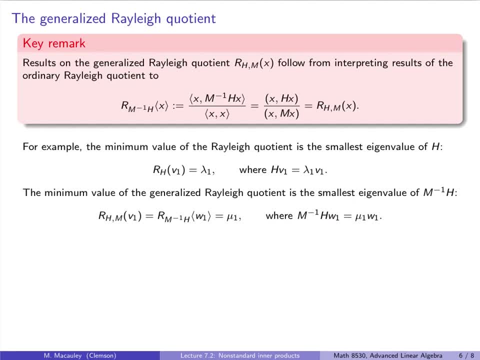 for some eigenvector v1.. And often this is written as hv1 equals mu1mv1.. Let's think back to what we did with the standard Rayleigh quotient. We found its minimum value and that occurred on an eigenvector. 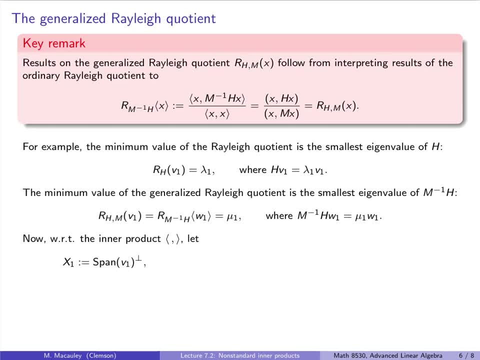 So we took the n-1 dimensional complement of that eigenvector, We called it x1.. So the complement of that eigenvector line, And then we found the minimum of the Rayleigh quotient on that space And that was the second largest. 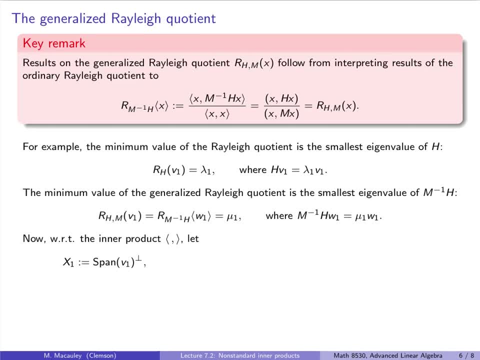 sorry, second smallest eigenvalue And we just iterated that process. So let's iterate that same process, but with a generalized Rayleigh quotient, which really is the standard Rayleigh quotient, with a different inner product. So x1 is the orthogonal complement. 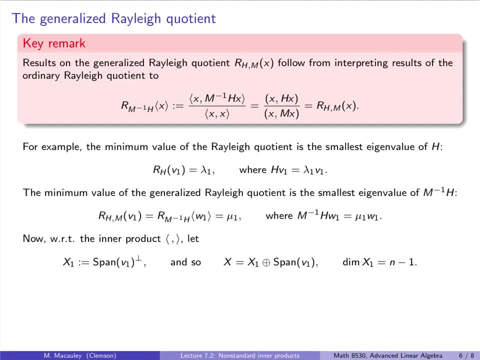 of this eigenvector. So x is the direct sum of this n-1 dimensional space with that eigenvector line And the minimum value of the generalized Rayleigh quotient on the subspace, x1, let's call it mu2.. It's the minimum. 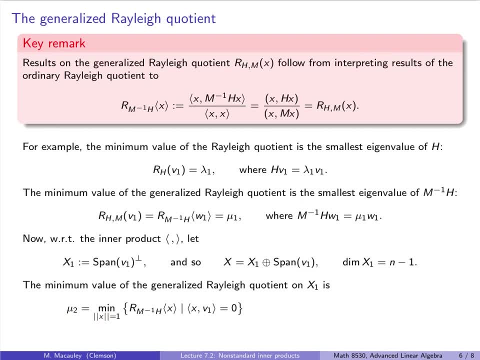 remember we only need to look at unit vectors over or of the function of the standard Rayleigh quotient with respect to this non-standard inner product, restricted to all vectors that are orthogonal to v1.. That's the definition of x1.. So if we interpret this back, 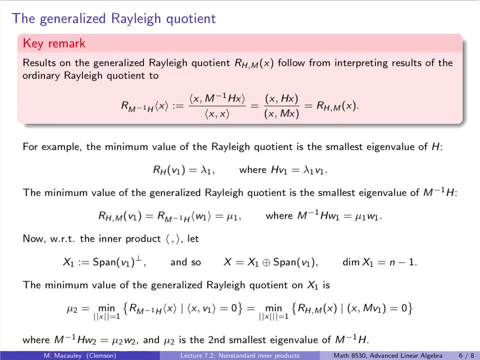 to our standard inner product, we get the minimum over all unit vectors Of the generalized Rayleigh quotient, restricted to all vectors x that are orthogonal to m to v1, m times v1. And here mu2, regardless of the inner product structure. 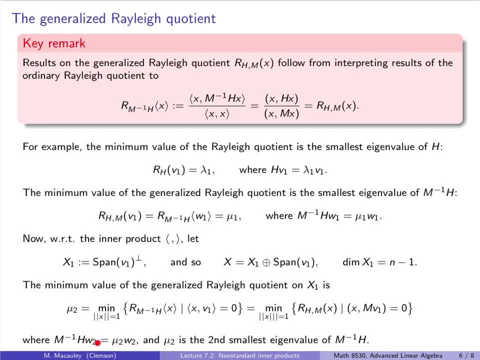 is an eigenvalue, say of eigenvector w2 of m inverse h. So m inverse h w2 equals mu2 w2, and this is the second smallest eigenvalue of m inverse h. Once again, I'm not proving this. 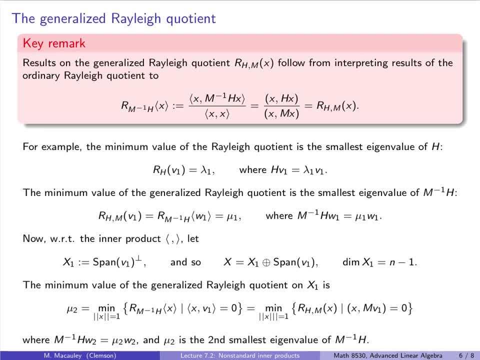 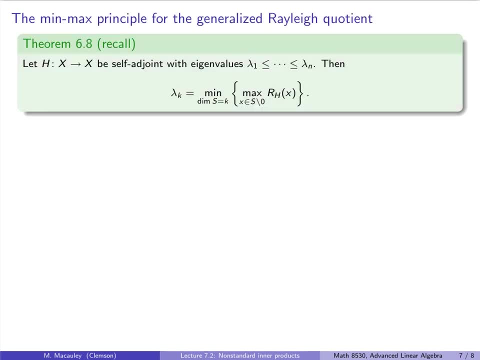 we did the proof for the standard Rayleigh quotient. I'm just interpreting the results in terms of the generalized Rayleigh quotient. Recall from the lecture on the Rayleigh quotient that we also had a so-called min-max principle. So if we had a self-adjoint linear map? 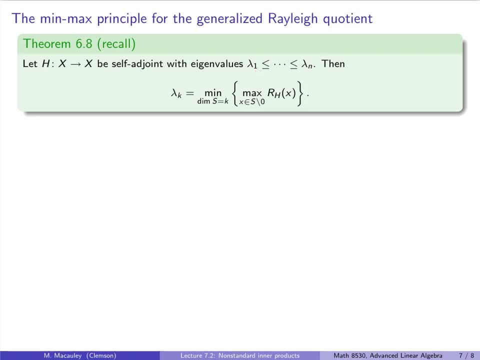 with eigenvalues, in increasing order, lambda 1 up to lambda n. then the kth smallest eigenvalue was the minimum, over all k-dimensional subspaces, of the maximum Rayleigh quotient on that subspace. So again, I'll refer you back to the original lecture. 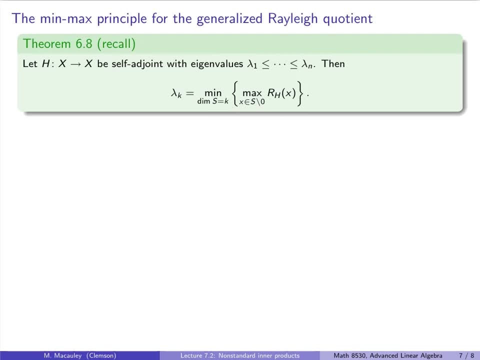 for some examples of this and some motivation. But let's now interpret what this says about the generalized Rayleigh quotient And I will leave the details as a homework exercise, Just like we did in the last slide. it's not really anything new. 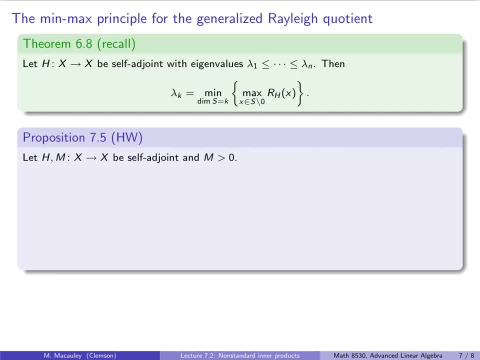 it's just interpreting our old results, So I will state them here. Suppose h and m are self-adjoint and m is positive, Then there exists a basis v1 up to vn of x, where each vi satisfies the following: 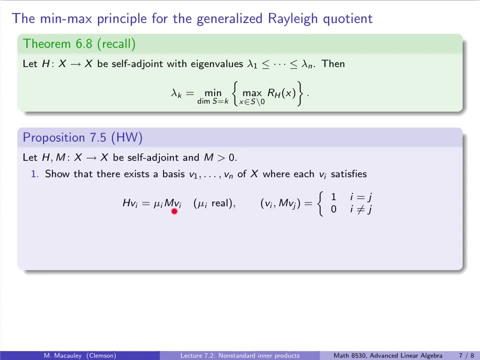 h vi equals mu i, m vi where mu i is real, and the inner product of vi with m? vj is 1 if i and j are the same and 0 if they are different. Now the reason why this is true. 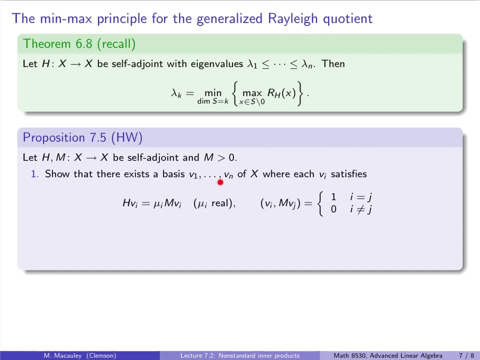 what this is really saying is that this basis is orthonormal with respect to the non-standard inner product. That is, if x and y, the inner product of this is x dot my, Because think about what this is saying. This is really saying that. 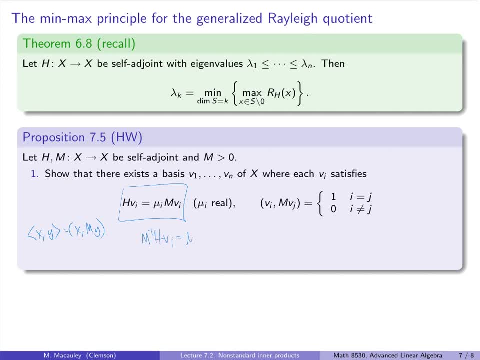 m inverse h. vi equals mu i, vi. So this is the basis of eigenvectors of m inverse h And this looks like on the right, it looks like the orthonormal condition and it is this right. here is just the. 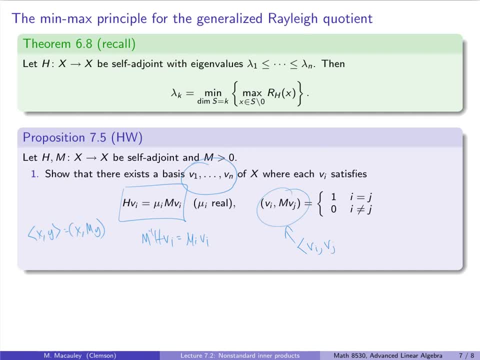 non-standard inner product of vi and vj. Also on your homework, I want you to compute the inner product of vi and h? vj. It might be easier to think of this as the in terms of the non-standard inner product of vi and m inverse h vj. 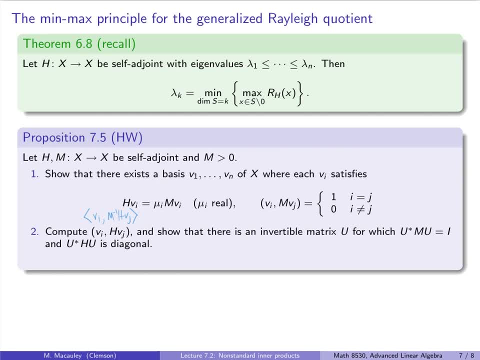 And show that there is an invertible matrix, u, for which u star mu is the identity and u star hu is diagonal. And finally, I want you to characterize the eigenvalues mu 1 up to mu n by a minimax principle like this up here: 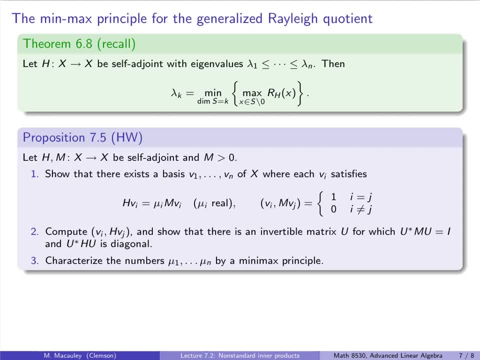 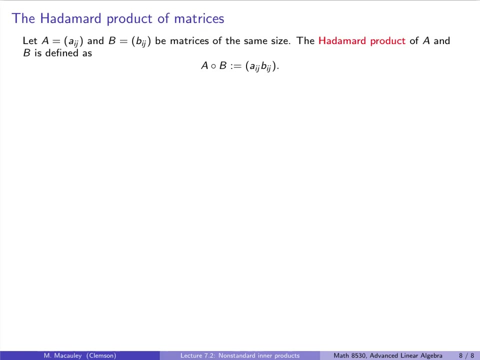 So again, don't reprove it, just use the existing one and interpret this, starting with the non-standard inner product, and then write it in terms of the regular inner product. I'll conclude this lecture with a surprising result about positive matrices. that really follows from. 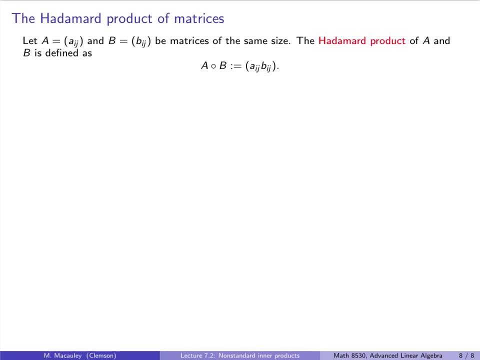 what we did on gram matrices. I put it at the end because I really wanted to not break up the flow about the non-standard inner products from gram matrices to the generalized Rayleigh quotient. So this is about the Hadamard product of matrices. 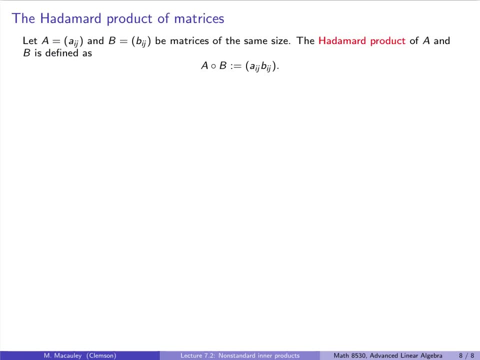 So if a and b are the same size, then imagine how someone who has never learned about matrices before is going to try to multiply them, Probably entry by entry. So if a is, say, a11,, a12,, a21,, a22,, 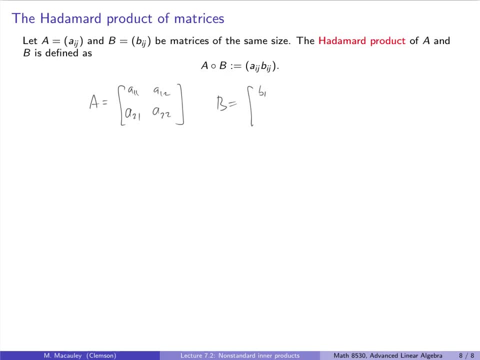 and b is b11, b12, b21, b22, then the Hadamard product of a and b is you just again, you multiply the corresponding entries, almost like you're taking a dot product. Well, it's not a dot product, because what you end up with 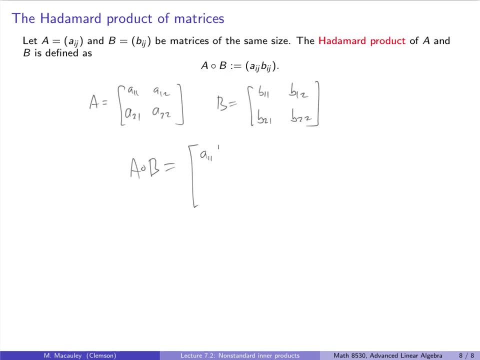 is not a scalar. Yeah, so it's a11, b11, a12, b12, a21, b21, a22, b22.. Shor's product theorem says that if a and b are positive, so they have to be square for that. 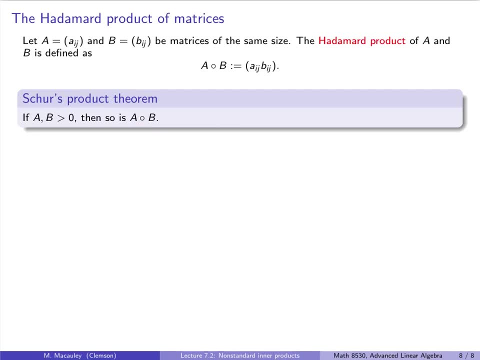 then their Hadamard product is positive as well, And this is something that you really should not expect. It should come as a surprise, Because it's not clear at all, in what we've done this entire class, what the meaning of this product is. 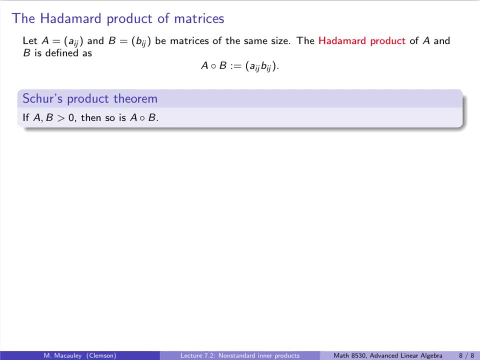 But the key here is to use the theory of Gram matrices. So since a and b are positive, they are Gram matrices. All we have to do is show that this matrix is a Gram matrix as well. So let's write a, which is aij, as a Gram matrix. 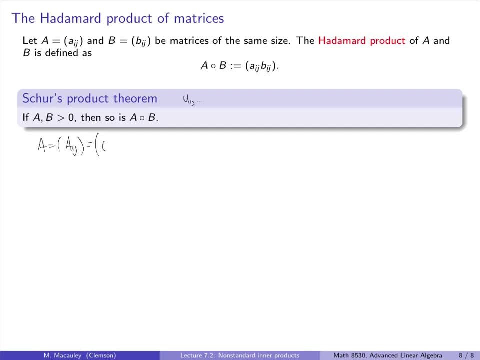 So we have some vectors- u1 up to um in the inner product space. u, So ui, dot, uj. I still like to write this. I like to visualize it like this: u1, dot, u1.. It helps me to see it like this: 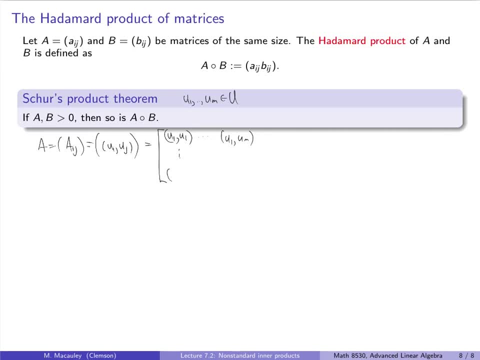 u1 um. Then we have um dot, u1, um, dot, um, Like this, And then b is bij. This is a Gram matrix. So in some other inner product space the inner product structure is generally going to be different. We have vi dot. vj is the ij entry. 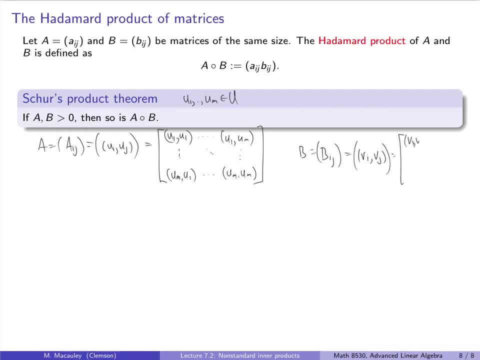 And so, once again, this is v1, v1, dot, dot, dot, v1, vm, vm, v1 and vm, dot, vm. I'm just writing this because I like looking at it. This is v1 up to vm in some v. Now I'm using the same notation for both inner products. 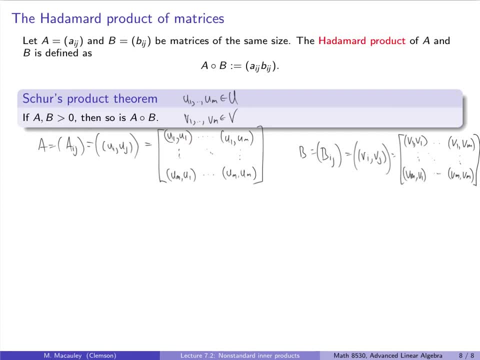 I think it's clear from the context. You know some people like to use this. One of them is brackets for one or maybe a subscript, u and v, But I think that would only make it just more messy. So the trick here is to consider: 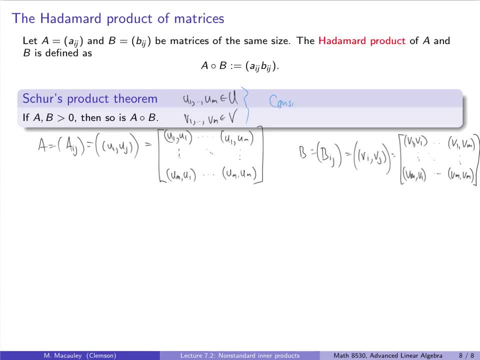 is given this. let's consider the tensor product. you probably didn't expect this to come up of u and v, And one thing that I have not said- I think I will in the future leave this as a homework exercise- is to understand what the inner product structure is. 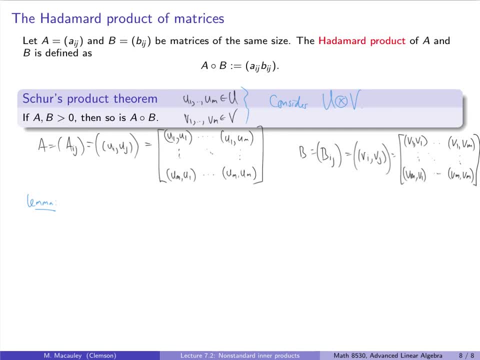 on the tensor product. So again, tensor products are fairly abstract. It's often helpful if you have ui, tensor vj. Sometimes it's helpful to think about this as, like x to the i times y to the j, You really are multiplying. 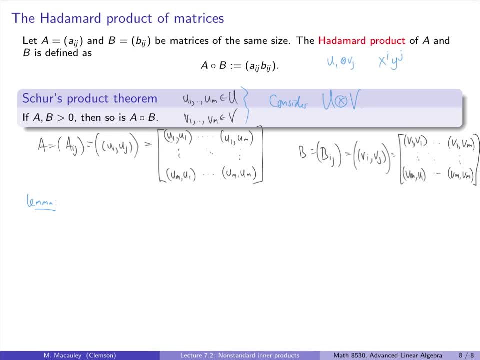 You're creating a new vector space where the basis elements are the products of things in here and things in here. So a lemma that I will leave as an exercise is that u tensor v inherits an inner product structure from u and v, where- and we can define it on pure tensors- 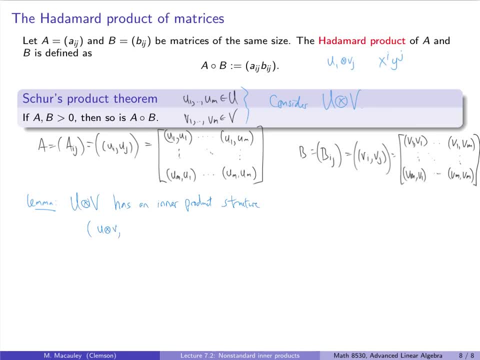 where the inner product is the structure of u tensor, v and u prime tensor. v prime is the product of u tensor. sorry, the product of the inner product of u and u prime and v and v prime. So you're multiplying. think of it like variables in x and variables in y. 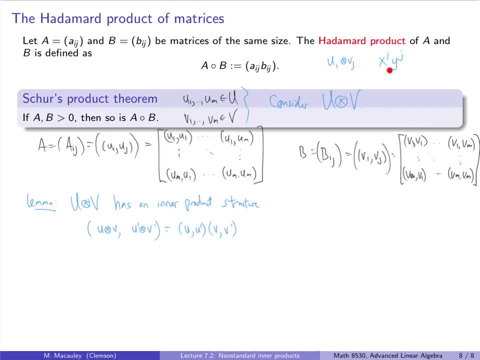 So, in terms of the inner product, you just multiply the corresponding inner products together. You've got to check that this works. I think bilinearity is the hardest thing to check, but the other properties, like symmetry, are pretty easy. Okay, so now what? 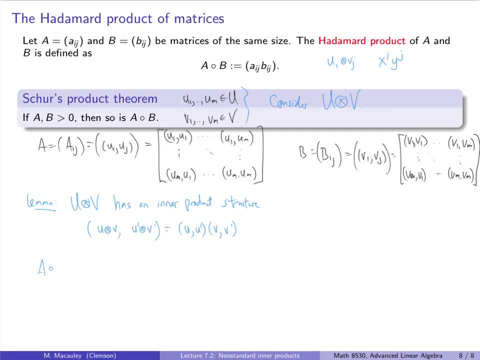 So we're trying to show that the Hadamard product of A and B is positive. So this is A ij, B, ij and that's just the product of ui dot uj and vi dot vj. So let me write that as. 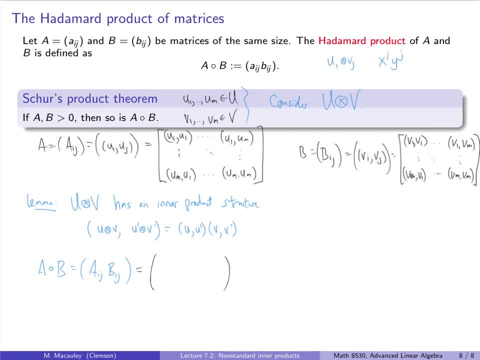 so that is the matrix where the entries are ui dot uj and vi dot vj. Now look at this definition of the inner product. here We can go backwards. We can write this as the inner product of tensors. So this thing right here. 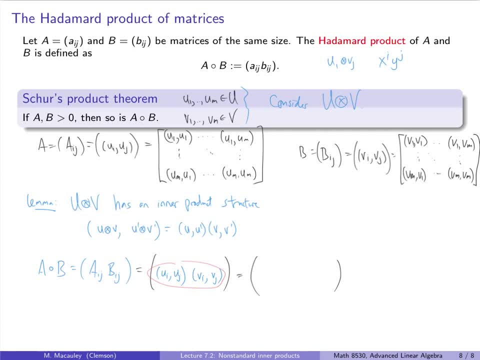 I'm going to write this as ui, tensor vi: dot uj, uj, tensor vj. I'm going to write it like that. And now we see right away that this is a gram matrix, So it is positive definite. And just to think about what this is, 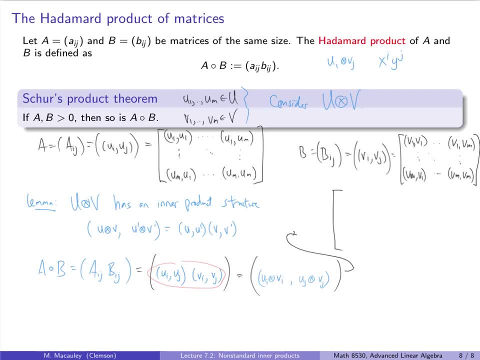 so this matrix is- I'm going to write it like this- g1 dot g1.. So what we've basically done is show that this is a gram matrix. So g1 dot g1, g1 dot gm, gm dot- gm.